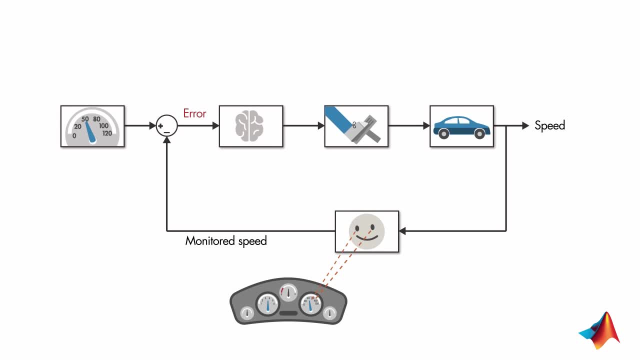 Now that we identified the components, we'll now talk about the control system. Once the control system is connected, the car will start moving. The control system will automatically. let's talk about how they are referred in control theory. In a feedback control system, the goal is: 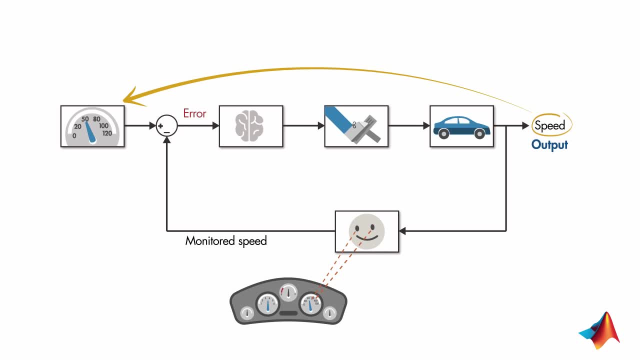 to control the output to a desired value, and that value is referred as desired output. Other common terms are reference and setpoint. The object whose output you try to control is called the plant. The output of the plant is measured by the component called the sensor, And the measured output is then. 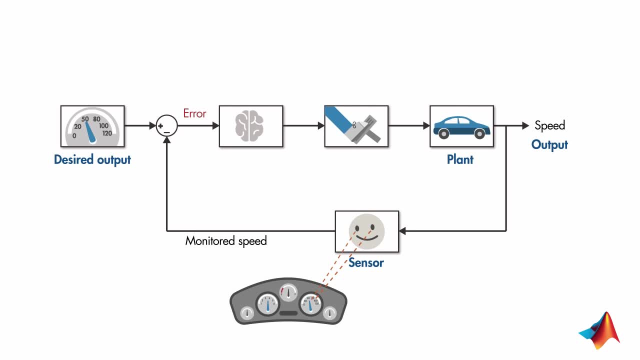 compared to the desired output. The difference between the desired and measured output is the error. Based on the computed error, the controller decides on the control action and it commands an input which is then sent to the actuator. The actuator is how. 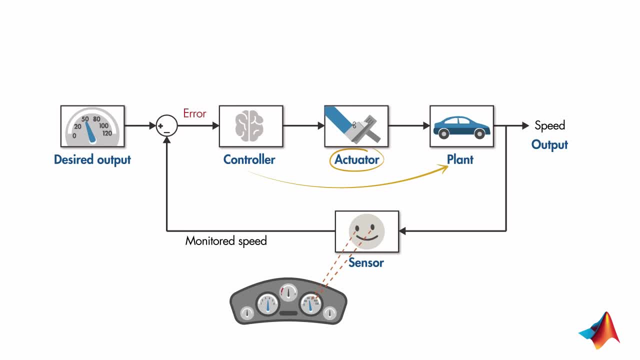 thisラ��은 control 수ей 짜고 shore controlルthis is JO, The Jeffery Jaguar. This controller influences the plant. In some situations, you'll see that the actuator, sensor and plant dynamics are merged into one and referred to as the plant. 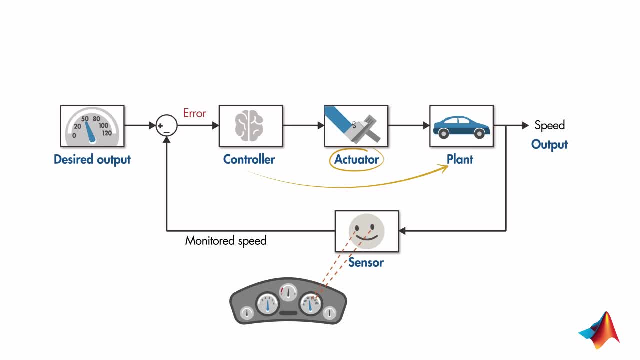 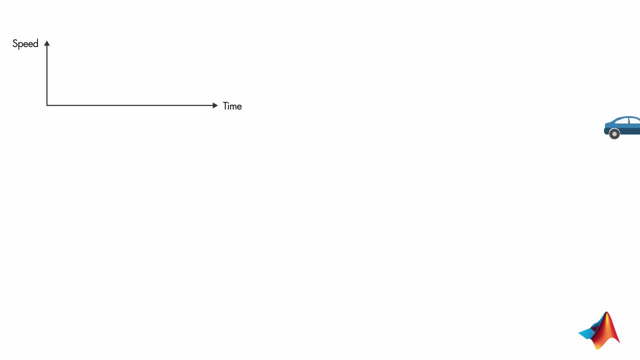 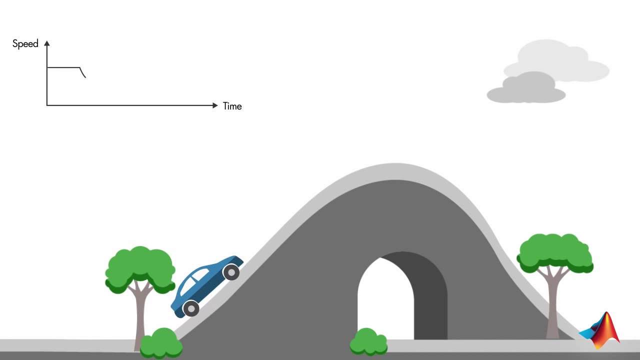 This may sound pessimistic, but life is far from perfect. Sometimes things may go wrong. For our example here, it is the road grade. Imagine you're going uphill. Your speed will start to drop due to the hill and you will need to press down further on the gas. 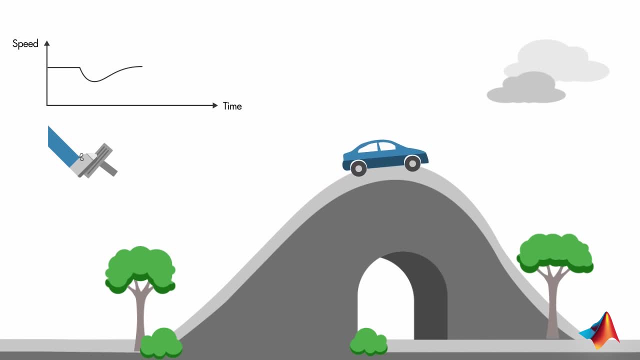 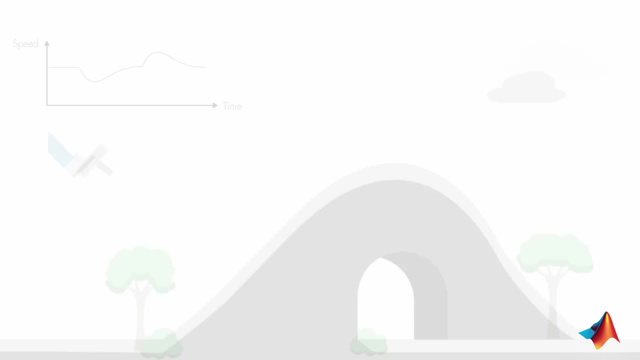 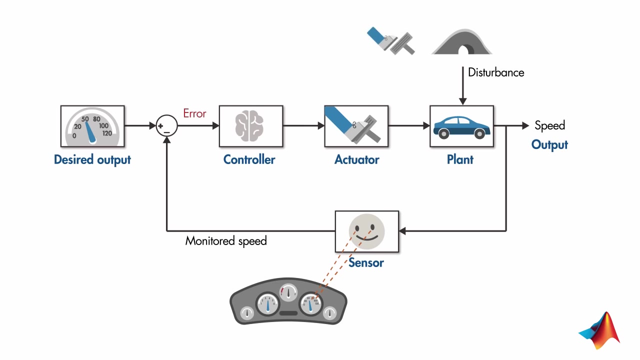 pedal to maintain your speed. Unexpected environmental changes causing the system output to behave in an undesired way, such as the road grade in this example, is called disturbance. Similarly, a sticky gas pedal, icy roads or windy weather act as disturbance on the car. 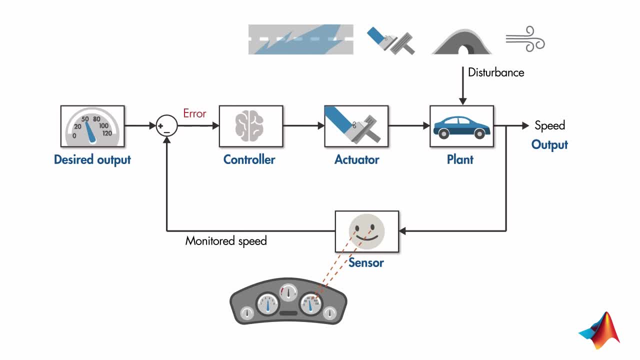 Another that may go wrong is related to measurement. While you're monitoring the speed- what if your vision is a little blurry because you forgot your glasses at home? The speed you're monitoring becomes noisy and fluctuates between values. This is referred as noise, which is an unwanted signal.